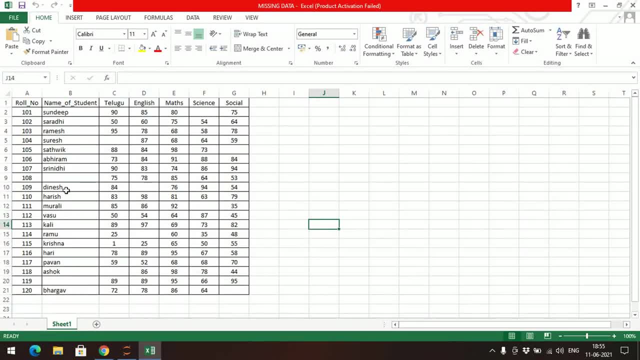 For example. so we are seeing the one example that is a mark of a student. So here you can observe there is some missing data. So in the name of the student, so two names were missing right And in the Telugu marks of a Telugu. I have just taken out two columns, I mean two marks. 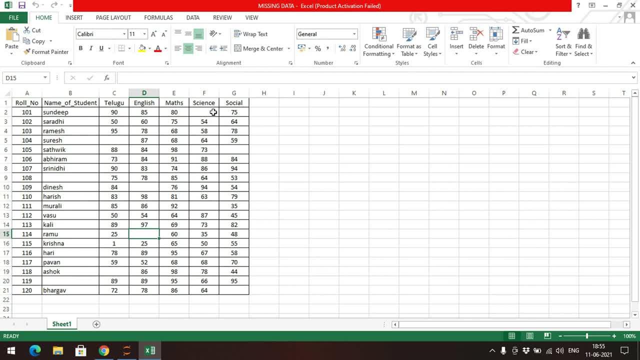 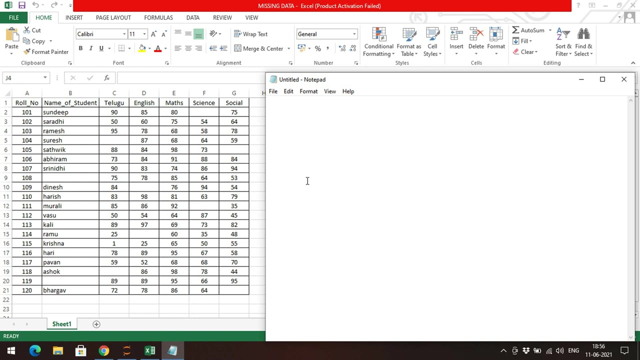 And here also some two marks are missing right. So like that, in the complete data set there might be some missing data. So how can we handle this missing data? So two ways to handle the missing data, So one is. so one way to handle it is remove- remove a missing data. 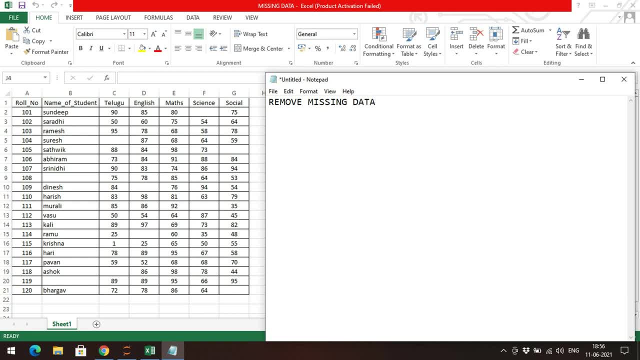 We can completely remove the rows which are having the missing data And one more fill the data fill with default values. So we can give some data So that can be filled with the missing data in case of missing data. So first we'll see this removing, So this can be done with the help of a function called drop an A. 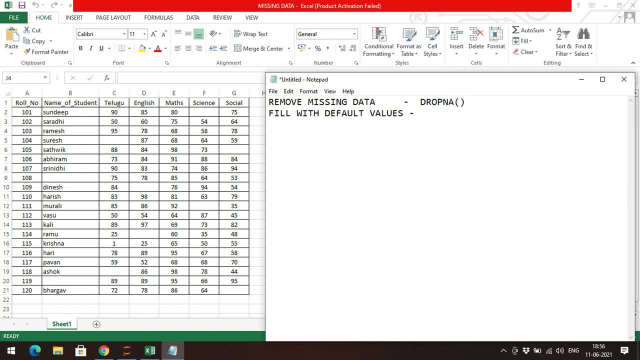 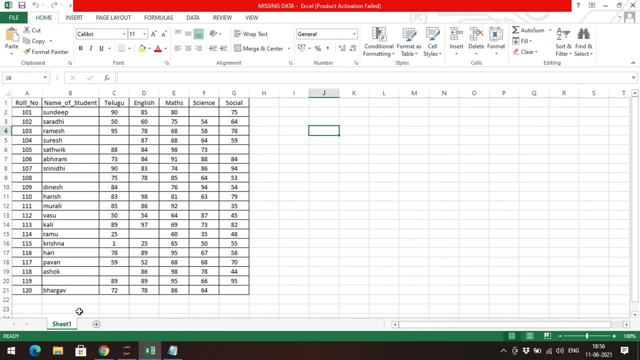 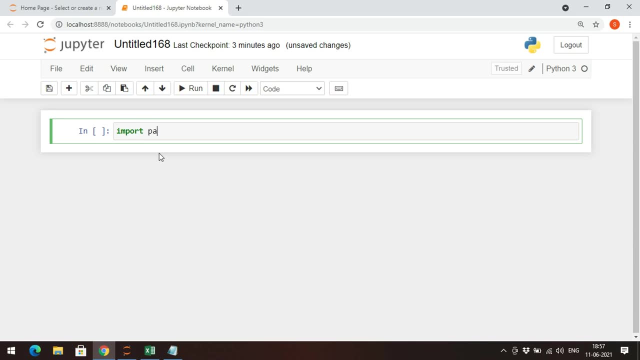 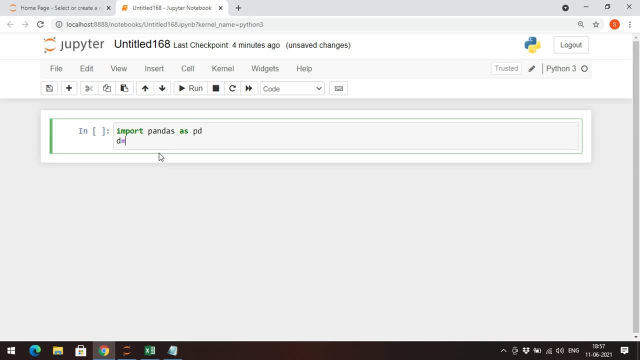 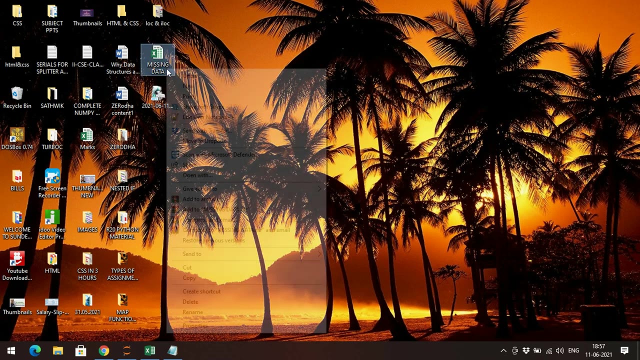 pd, so i am giving some alias name so that we need to read, with the help of this one, pd dot. read excel, read excel. so here we need to pass the location of that particular file. so i will pass the location of this file. so just go to the properties and there you can find the path. so just copy the path. 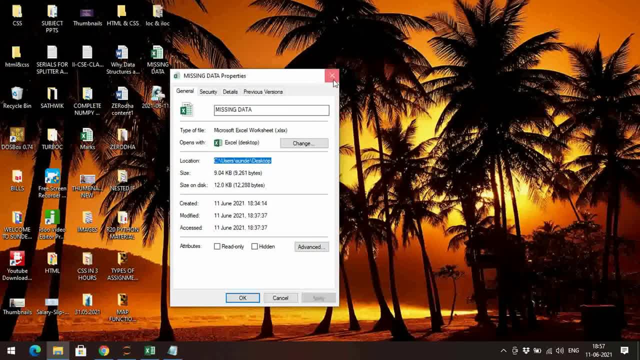 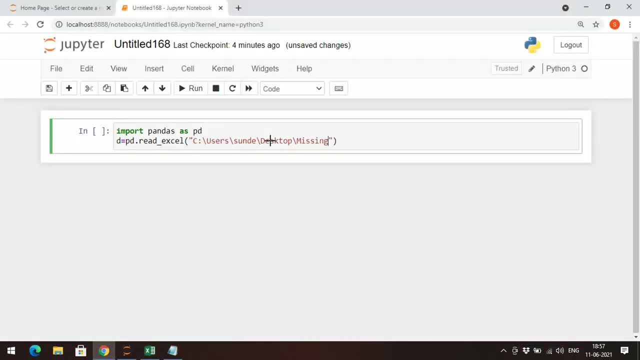 and paste the path in the location. right, see, i am just copying it and i'm pasting it. so here we need to give the yeah capital letters. missing data: dot, xlsx. so use the double flashes in the location. so this is common. we need to read: 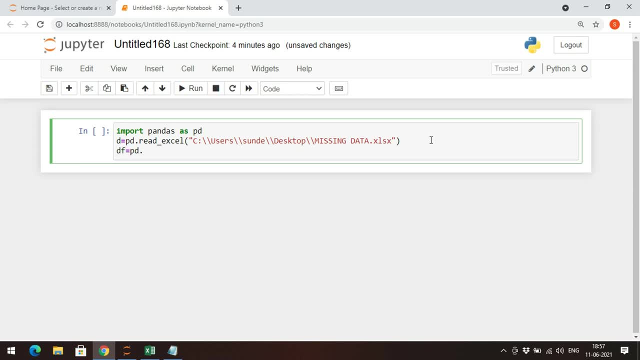 the value. and then we need to create a data frame at the df is equal to pd dot data frame and just pass the d as an argument. so so, implementing these three statements, executing these three statements, you will get the value of the data frame and then you will get the value of the data frame. 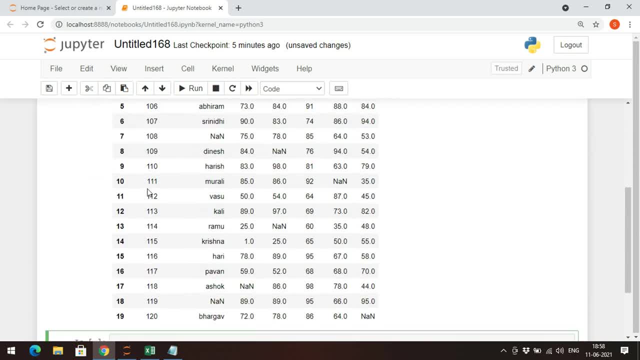 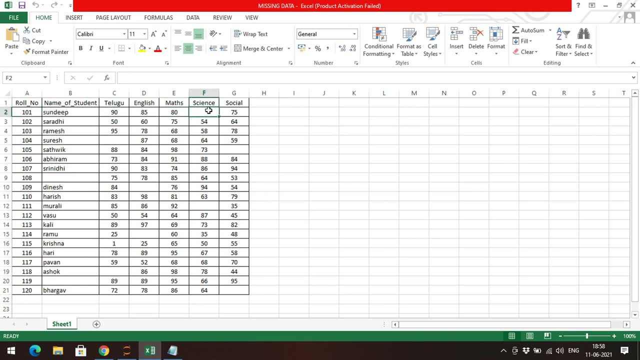 you can create a data frame. you can observe the df, so it's a data frame with complete data. you can get complete data. so here you can observe the missing data. so for example, in 101 roll number the science value is missing. so you can observe here 101 roll number science value is having some 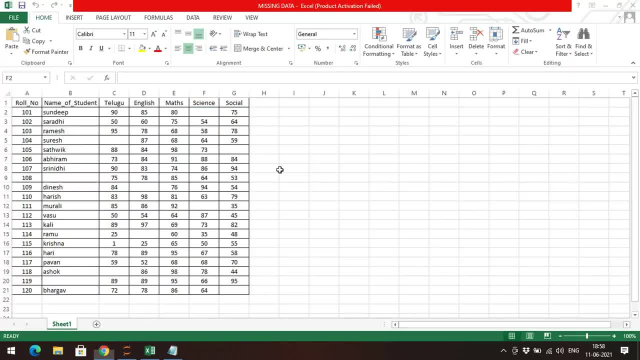 n a n. n a n means not a number, so all the missing data will be filled with this n a n. to raise 104 say n a n, and again so topic: social. so here you can observe n? a n right. so here some names are also. 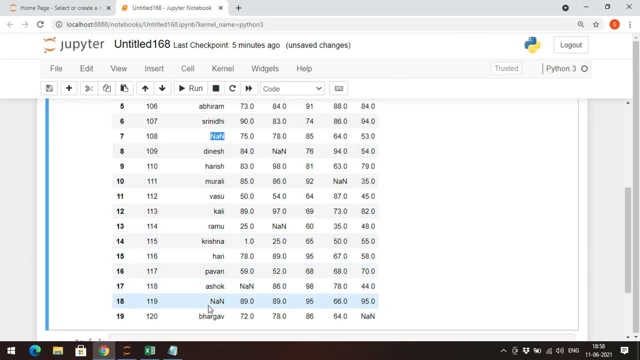 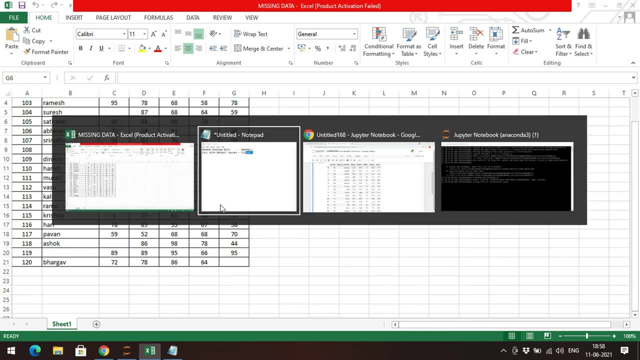 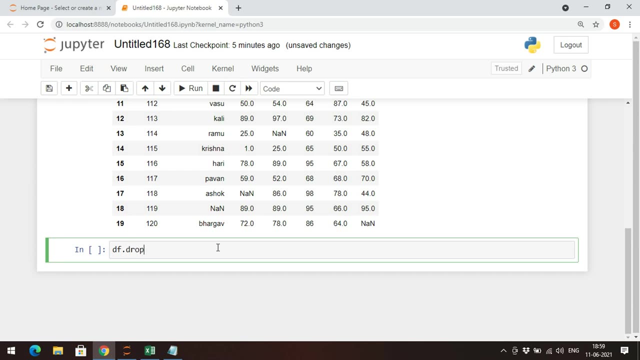 missing. you can observe here. so this name is missing here and here also a name is missing. so how can we handle this one? so first one we are, we have seen is that is removing missing data. so simply we can remove the missing data by using the drop n a. so df dot drop n a will completely remove. 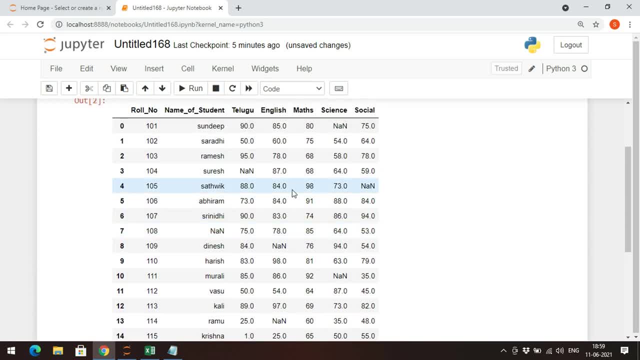 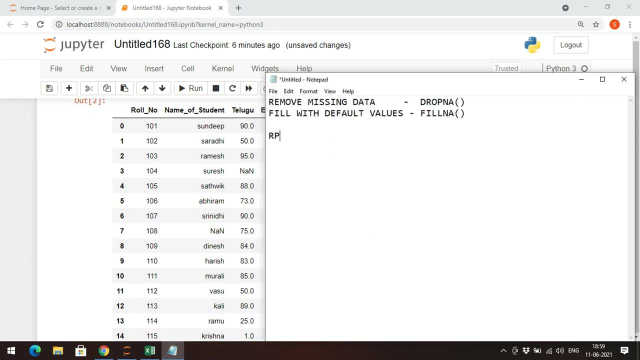 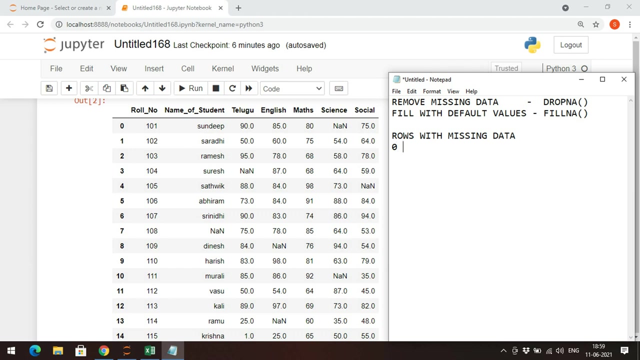 all the rows so you can remember the rows which are, i mean having the missing data. so you can observe here the rows, rows with missing data. you can observe here. so what are the rows, so we can see. so zeroth row, zeroth row, and we can observe here the third row and fourth row, and seventh row, eighth row. 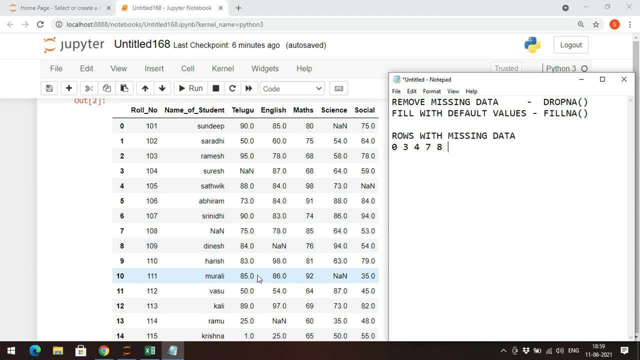 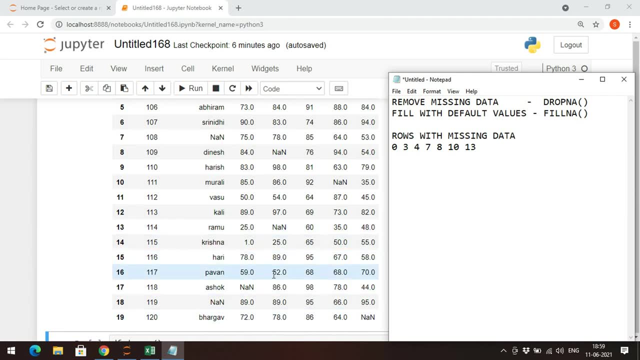 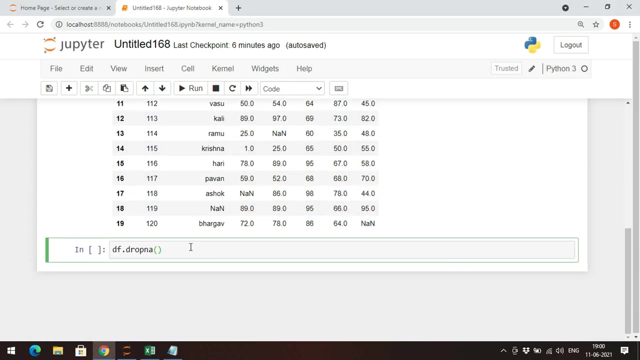 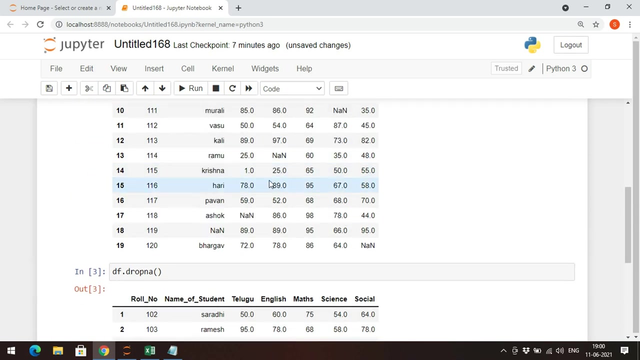 tenth, thirteenth, eighteenth- sorry, seventeenth, eighteenth and ninetieth. okay, you can observe. total 10 rows are there with missing data, 10 rows. so if you execute this one, if you execute with a drop n a, so you will get only the 10 rows. so all the rows which with which are having the missing values will. 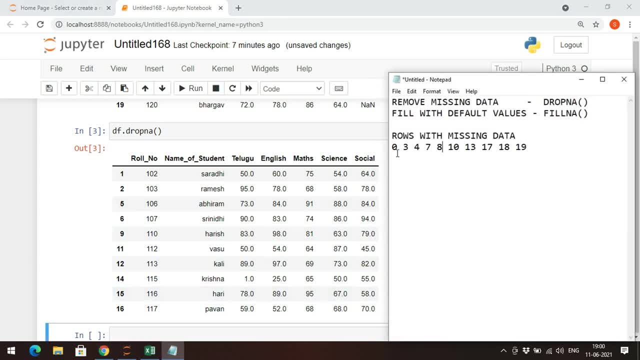 be removed. okay, you can. you can observe. we have noted out zero. there is no zeroth row. third: third row is missing. fourth: they're not there: seven, eight and ten, thirteen, seventeen, eighteen and nineteen. so all these rows are having the missing data. so all the rows have been removed. and one thing you need: 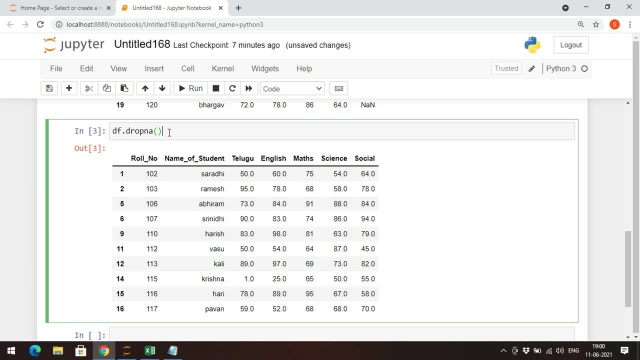 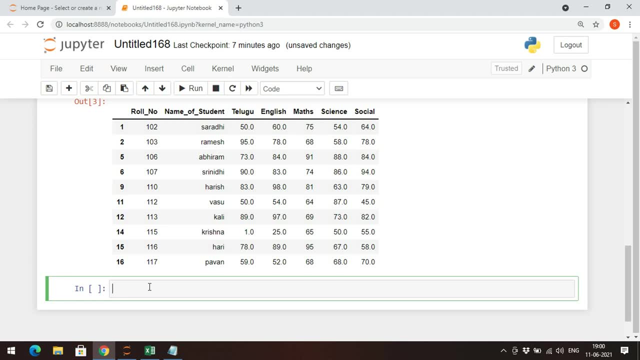 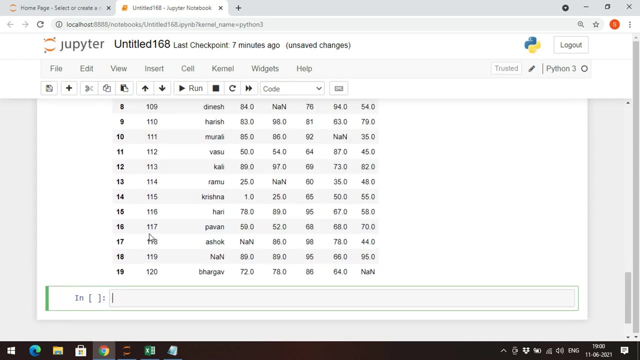 to observe is so this drop n a function. if we execute this drop n a function, it will create a new data frame, but the original data frame will not be affected. so still, after executing the drop n a, if you observe d, f, d, f, so you will get all the 20 rows. still, you are getting all the 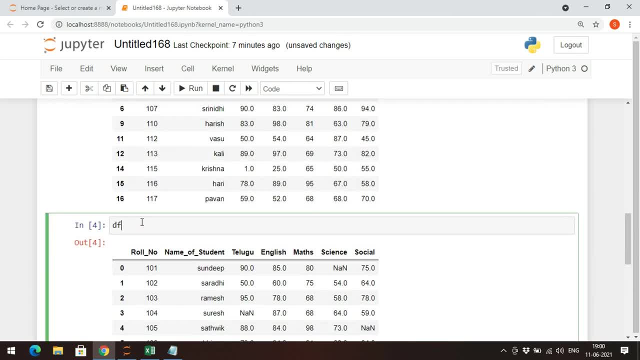 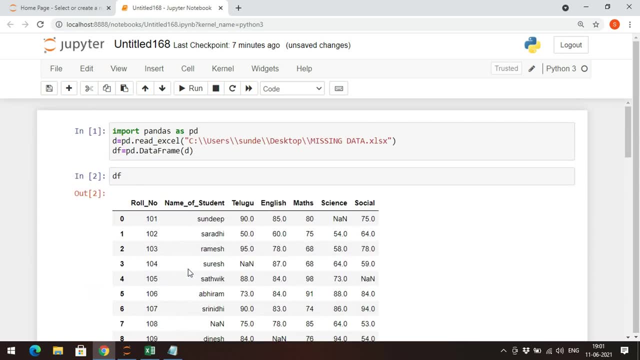 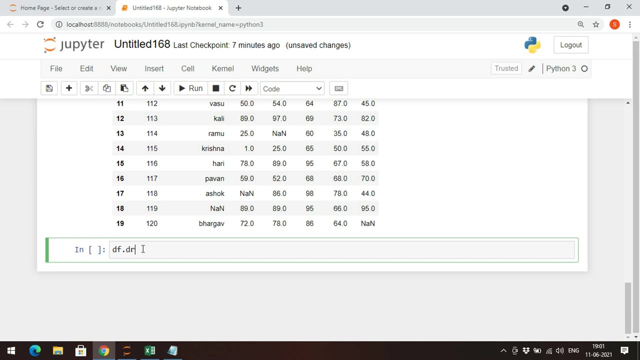 20 row, right. so this drop n a function will only creates a new data frame. so if you want to reflect the original data frame, just you take the parameter called in place. so d f dot, drop n a and give the parameter in place is equal to what you want to do. so here here: d f dot n a and this is the. 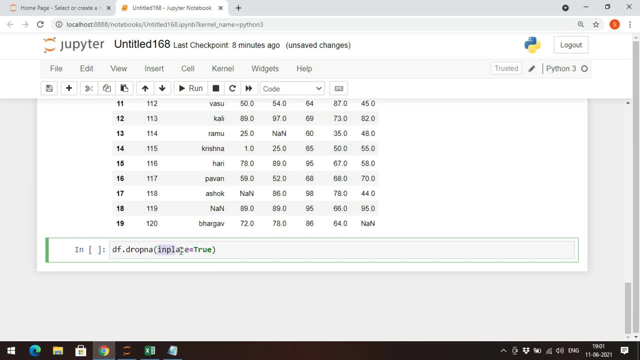 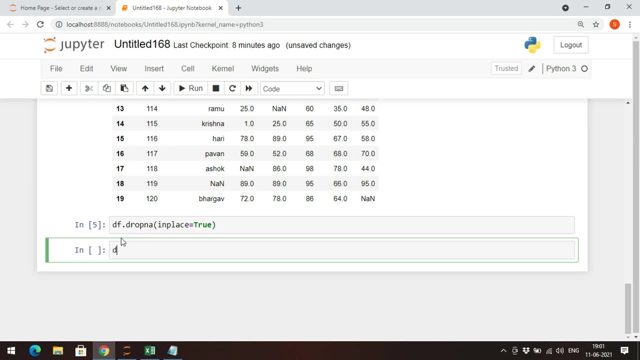 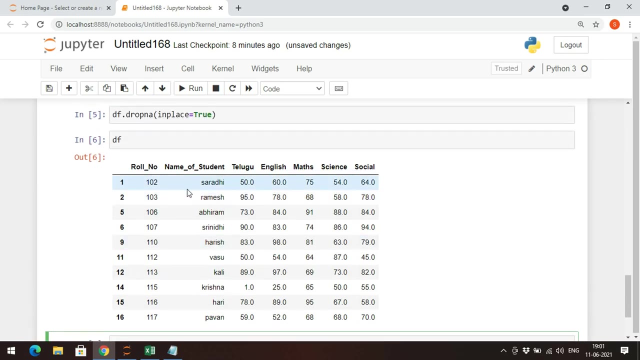 to true, so by default it will be false if you use this parameter in place. true, so the original data frame will be get affected, if you observe here. so nothing is displayed here. if you go with the DF, then we will get the new data frame without the missing data, right so previously, if you execute this one. so 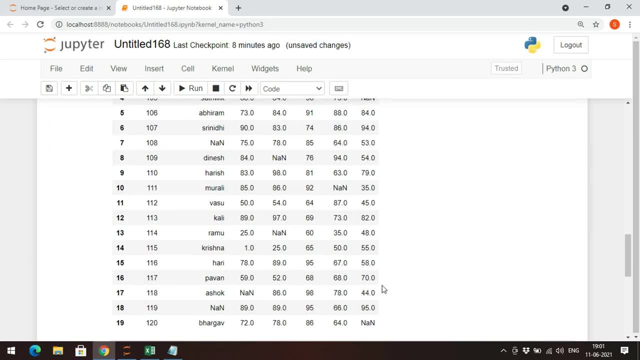 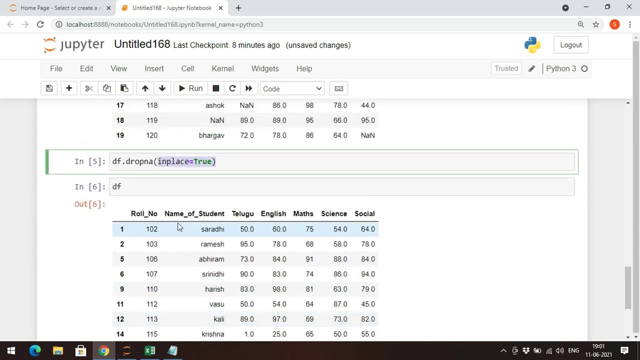 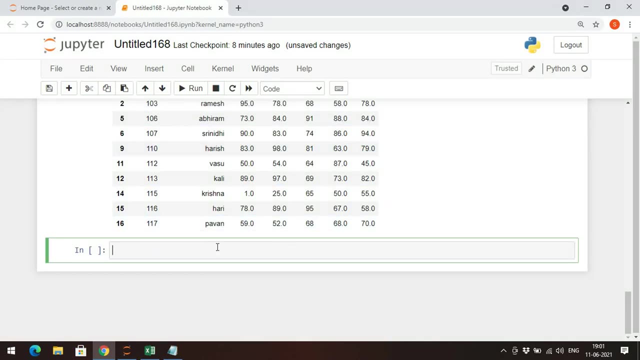 we will get the new data frame, which is not saved. okay, but if you use this parameter in place, is equal to true. the original data frame will be affected. okay, original data frame will be affected. right, see, once again, I will execute the same thing because our new data frame is not having any missing. 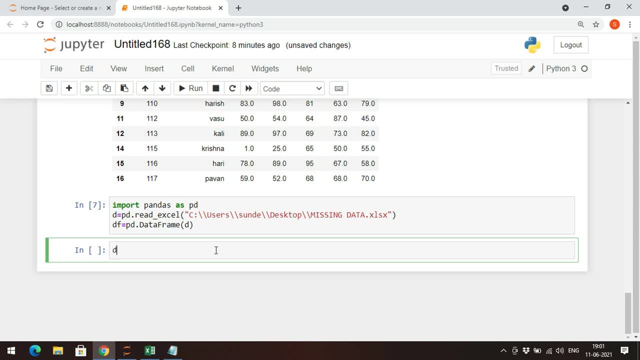 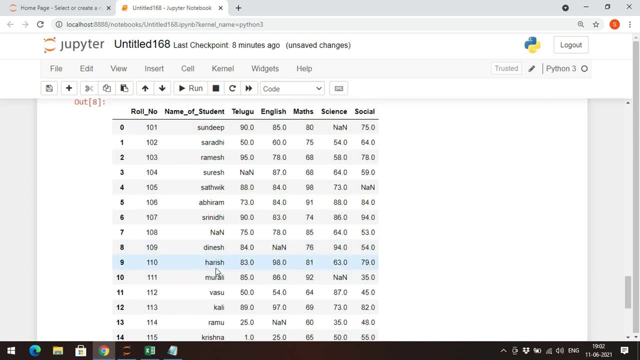 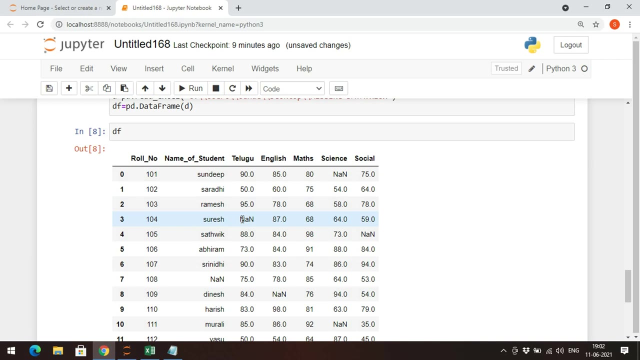 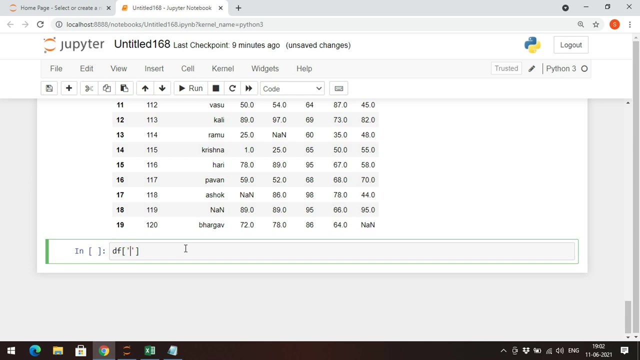 values because we have completely deleted all the rows, right? so if I go with the DF, I am having again 20 rows now. if you want to remove, okay. if you want to display only a particular column, with removing all the values, just go with DF, and we have seen how to access it. see, let us check with Telugu, so go with. 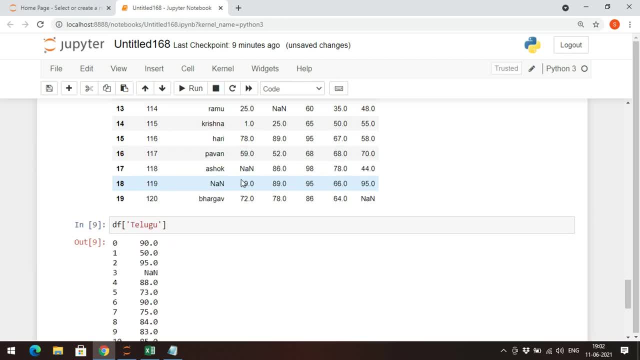 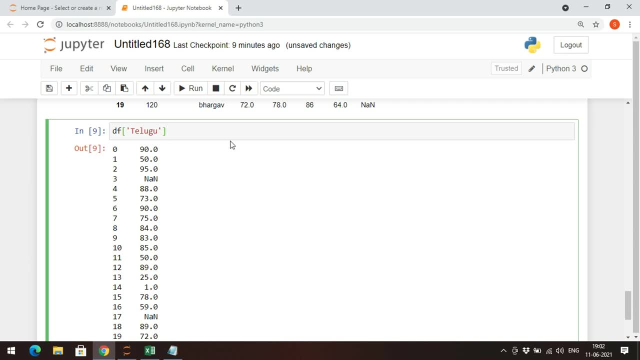 Telugu, so that it will return all, only the Telugu values. it will return only the Telugu values. you can observe here. right, so if you use the same thing, dots drop NA, it will return only the values. okay, without missing value, without the missing data. okay, you can observe here. 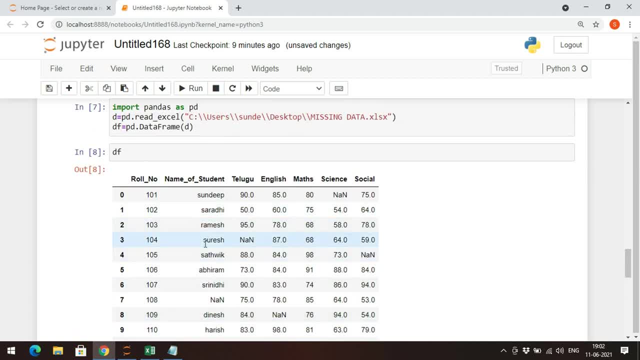 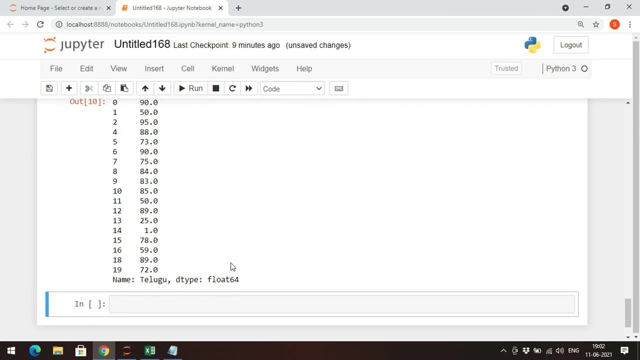 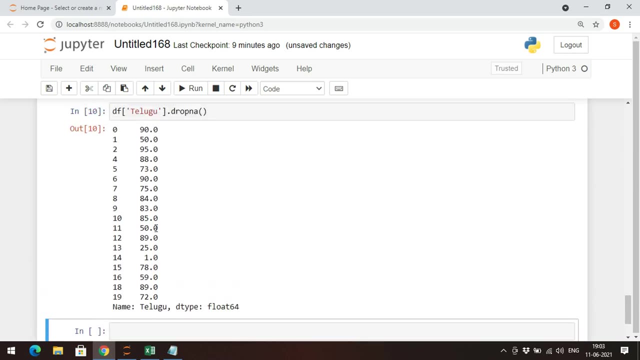 the Telugu marks. so we are having the third row. okay, 104, student. the data is missing here and similarly, 118 student- data is missing here. okay, and you just remember the row numbers 3 and 17, you can observe we will not get the third. 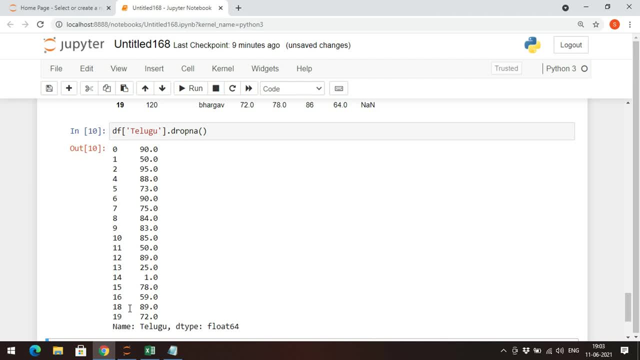 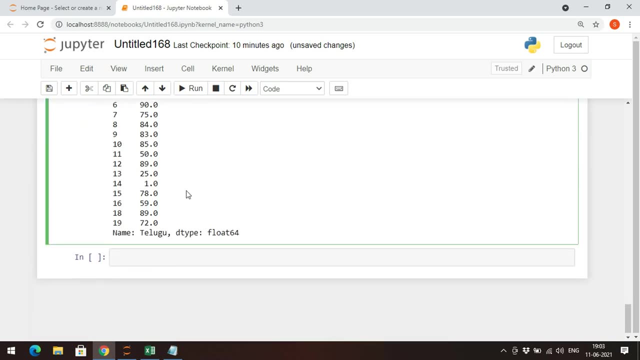 row and 17th row here. third row and 17th row right. so like this we can use the drop in here, or else, if you want to delete this missing data from two columns, you go with our LOC, which we have discussed in the just previous. 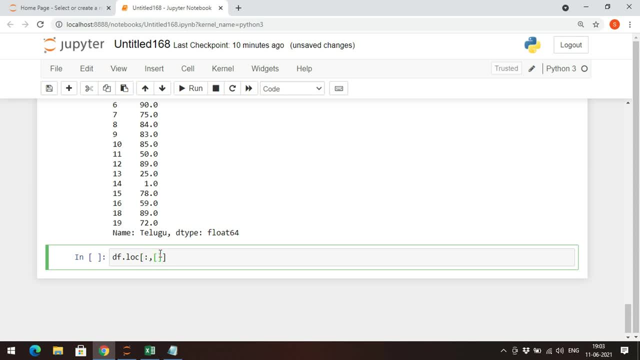 session. so go with all the rows and check with the columns, with the two columns, I will go with the two columns, so that is some Telugu and English. let us take some Telugu and English, so Telugu and comma English. so you will get only the data. see, you can observe only the. 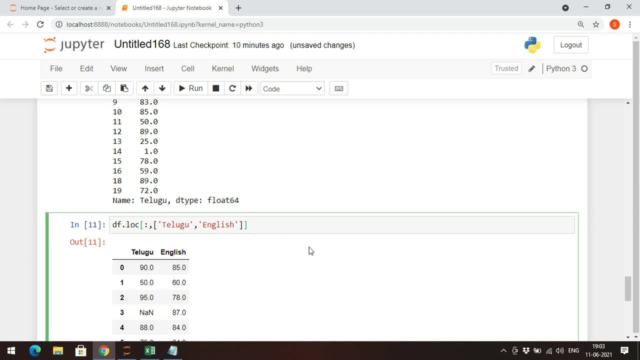 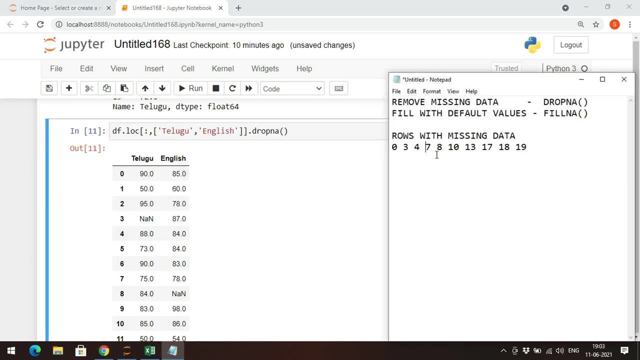 Telugu and English data we are getting. so if you use a drop in here so you can observe the row numbers, see here. we will write missing data in Telugu and English. you can observe the row numbers: see here. we will write missing data in Telugu and English. 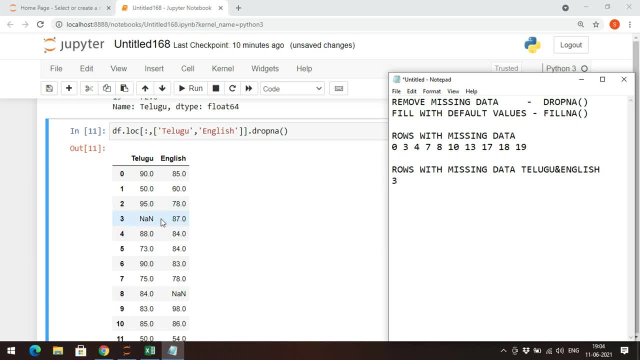 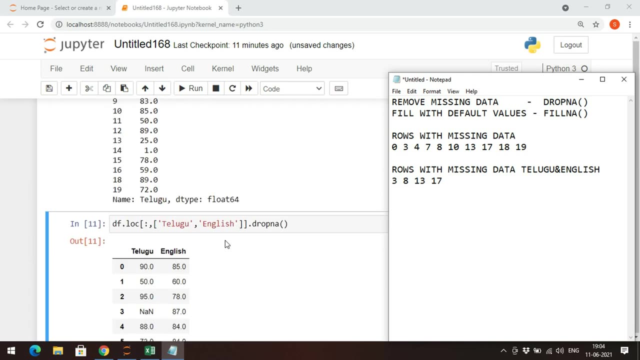 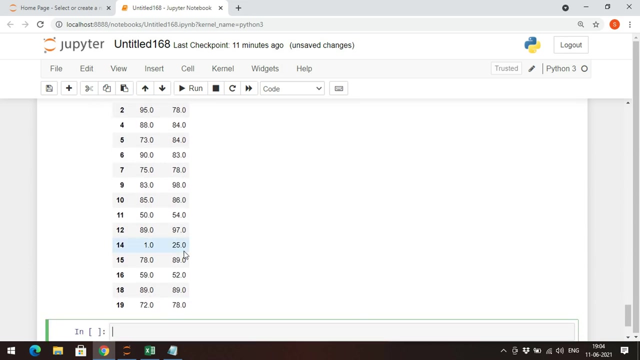 so you can also here the third row and 8th row and 13th Row and a 17th row, like so there are four rows with missing data. so if you execute the same thing, if you execute the same thing, see will get all the data without the missing data. so you 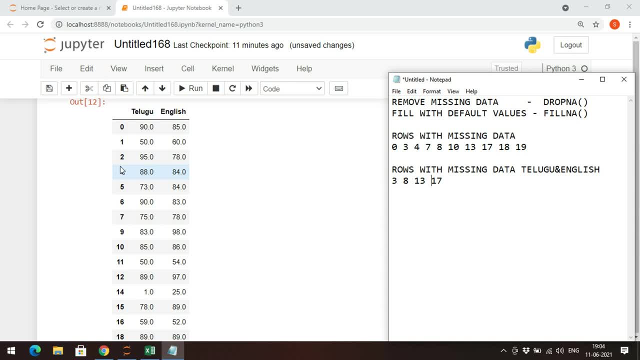 can observe here: third row, which was missing, completely deleted, and 8th row, which was missing, completely deleted row. it was deleted. 13th row was deleted and again 17th row was deleted because all these rows were having the missing data in both the telvi and english. you can observe here. so like this we can. 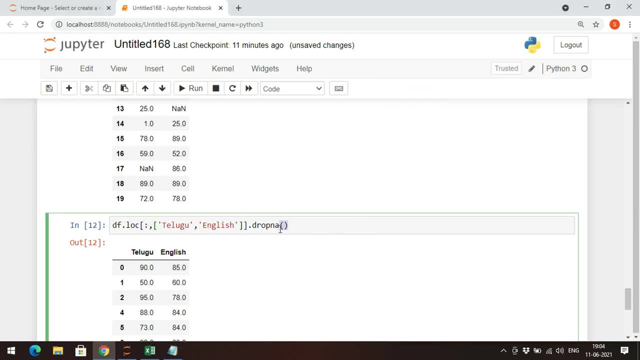 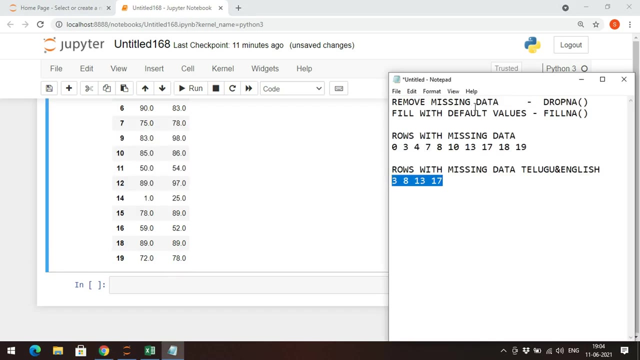 apply the loc option and the drop in here. so by using this one we can drop it, and if you go with this in place is equal to true. the same will be reflected with the original data frame, right? so this one option, this is one option to handle the missing data. that means directly removing the 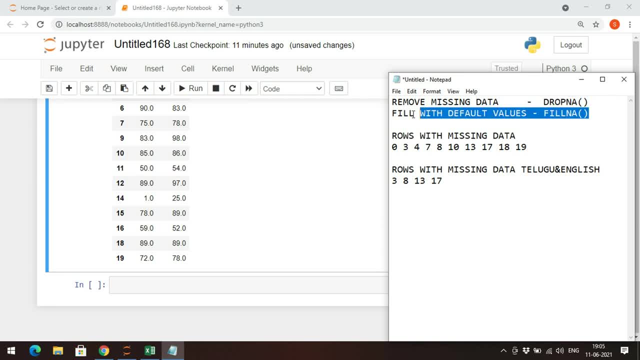 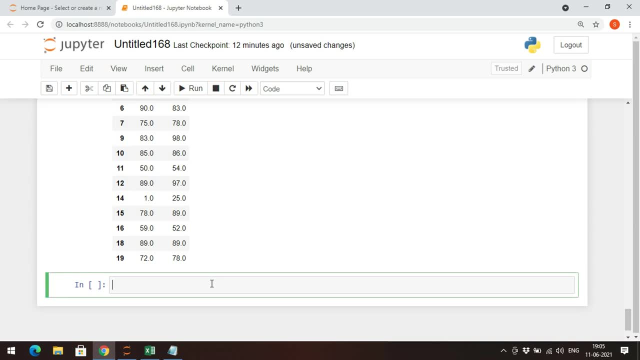 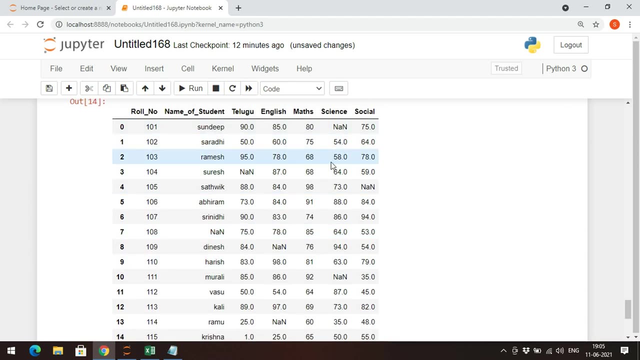 rows which are having the missing data and the next one is filling with the default value. so without removing, just filling with the default value. see, i will go with the df. sorry, it's a small letter, so df. so here we are having some data with the missing one. so if you fill with any, 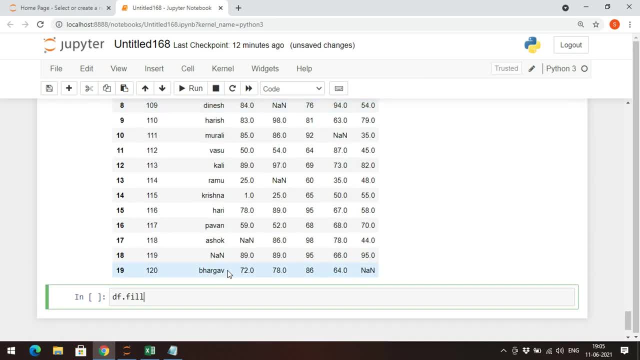 default values. we have to go with the df, dot, fill na and give the value here. so what is the value you need to give? okay, see, i will. i will write as missing. i will write as missing, so and just enter. yes, you can observe. so wherever the 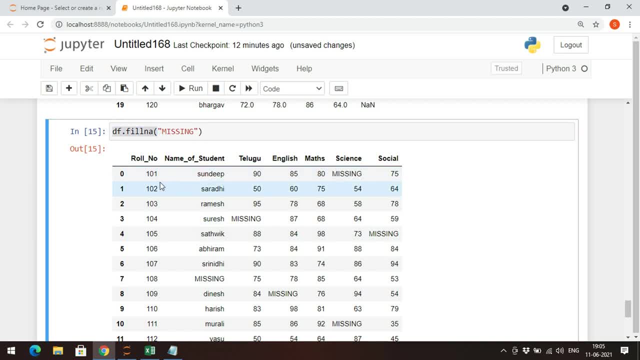 data is not available there. you can find the missing right: see 101 sandeep the science marks were missing and 104 furesh telugu marks are missing. 105 satvik social marks are missing. 108 the name of the student itself missing right. so like this. 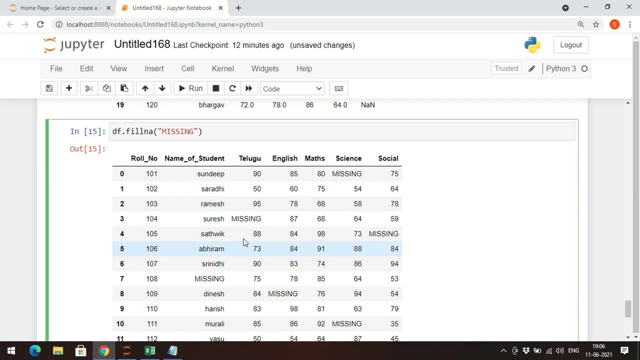 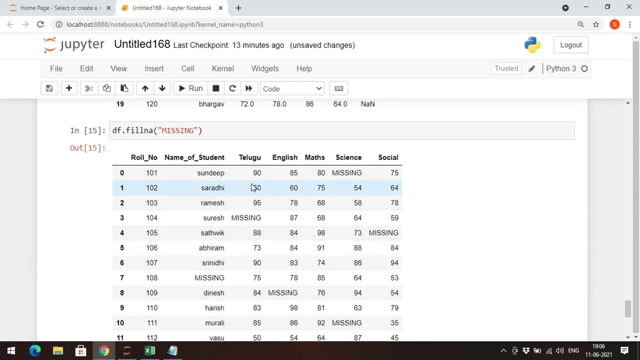 wherever we want to get the default value. there you can observe here. there you can write the data. okay, so if you want to give the marks for this particular student, okay, this one only. only give the default values for telugu. okay, only give the default values for telugu. 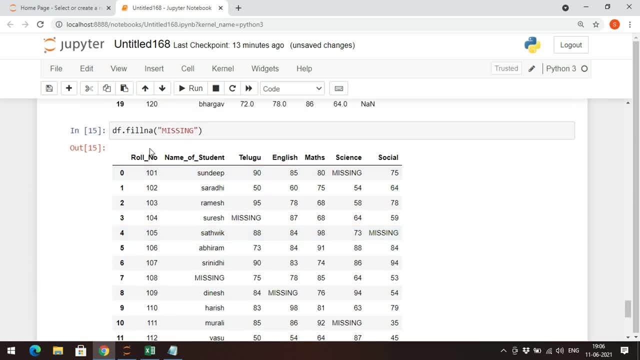 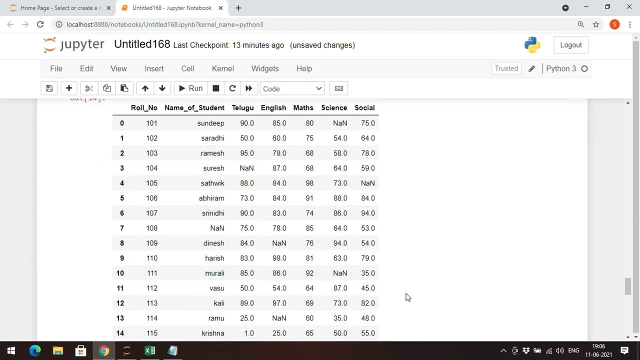 so here also, the original original data frame will not be reflected. it gives the new frame, and if you give the parameter as in place is equal to true, then the original data frame will be affected. so you can observe: original data frame will be affected. okay, so we can just go. 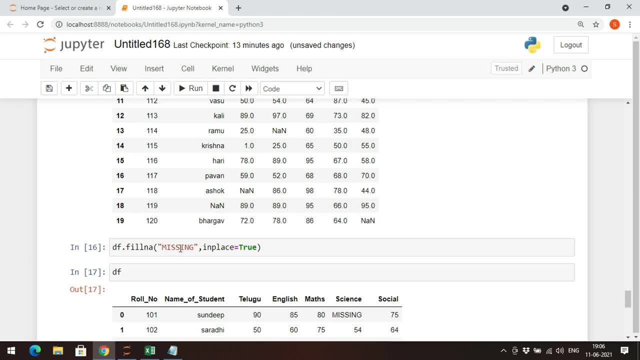 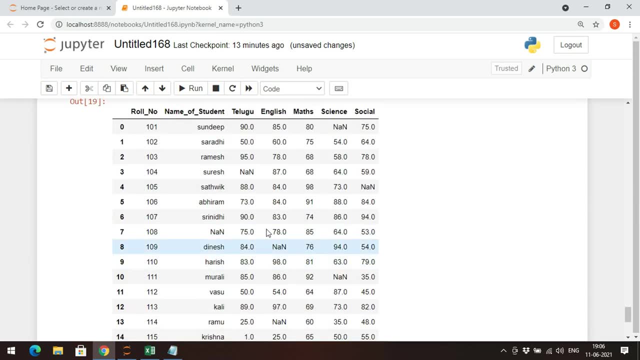 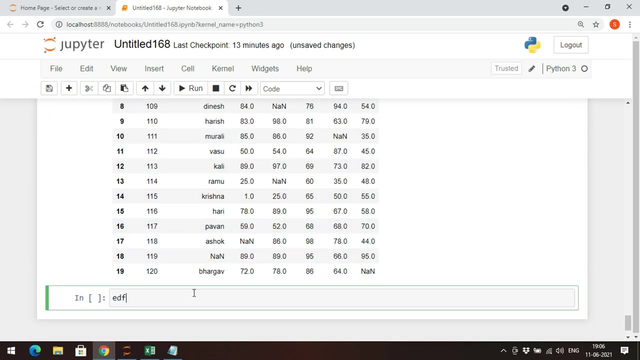 with the. once again, we will execute the same state of statement, because we need the data with the missing values, right, see df. so we are having some missing values, nan. so i just want to fill the default marks for telugu. okay, the students who are whose marks are missing. so i will go with a df dot. sorry, df of telugu, dftelugu. 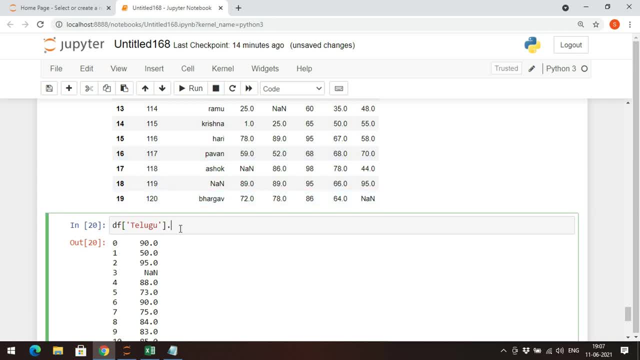 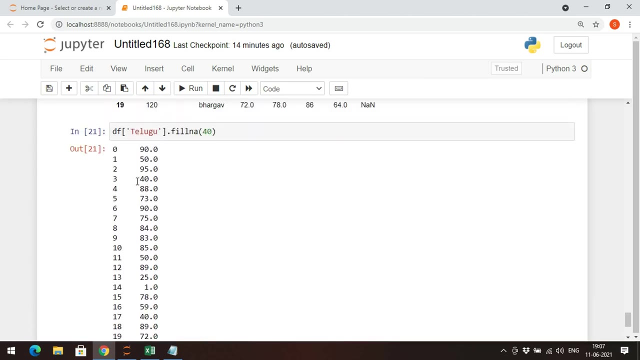 and if you observe, only the marks will be displayed and here you can observe, fill na and give the marks here. so let it be some 40 marks so you can observe whatever the missing telugu data. so third row and 17th row you can observe third row is filled with 40. that is the 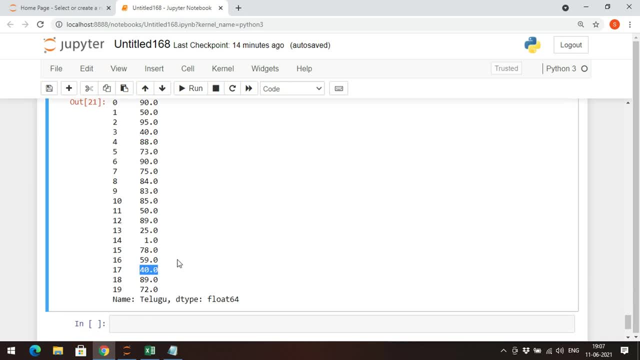 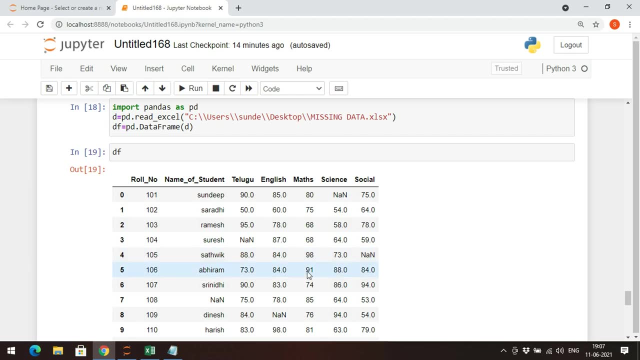 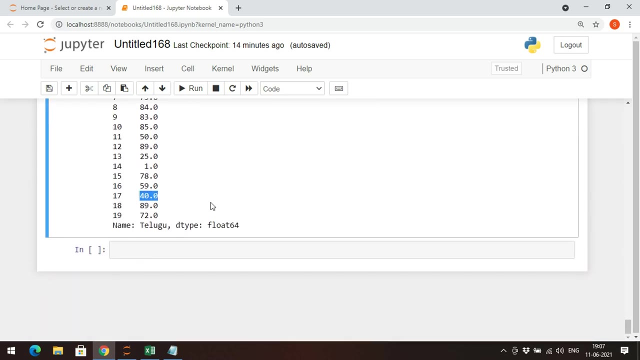 value we have given, and 17th row also filled with 40.. okay, so like this we can apply the missing data, right? so, similarly, similarly, if you want to fill with a different one, right so? df dot loc. i take the two columns, so go with the rows, all the rows, and go with the particular columns, so telugu. 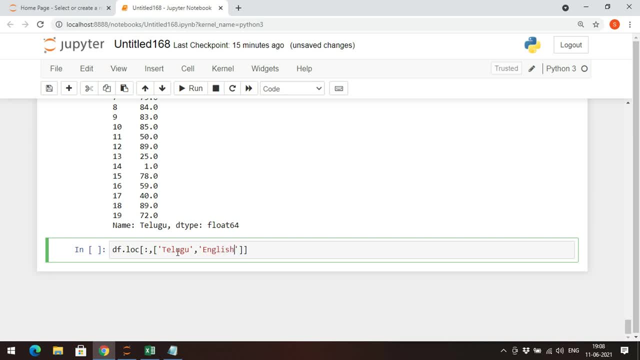 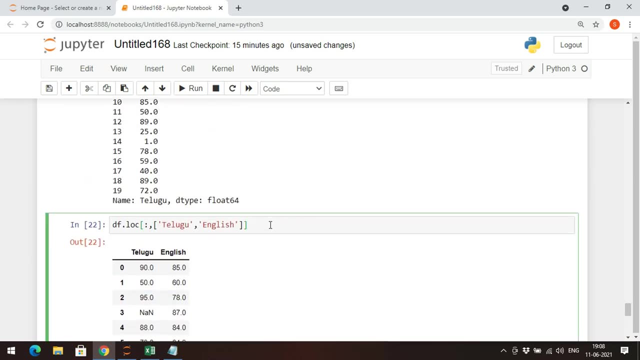 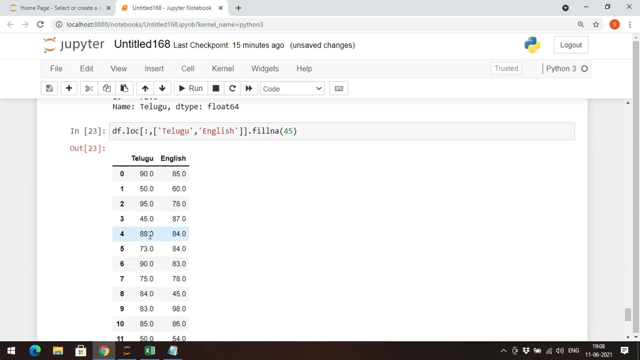 comma english, telugu comma english. so if you enter so automatically we'll get all the values. so here you can fill with a fill na of some 45. so automatically, whatever the values we are having. so you can observe here, see telugu in english: the third row. third row, we are having some 45, and eighth row: 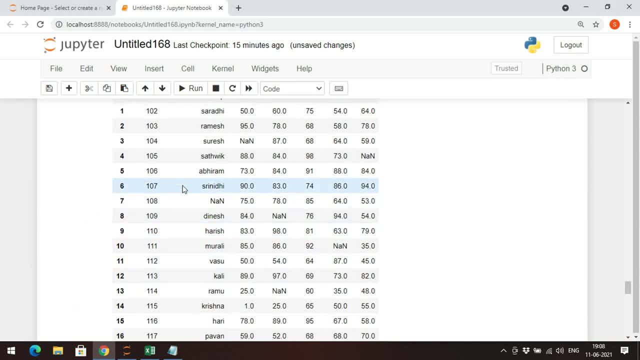 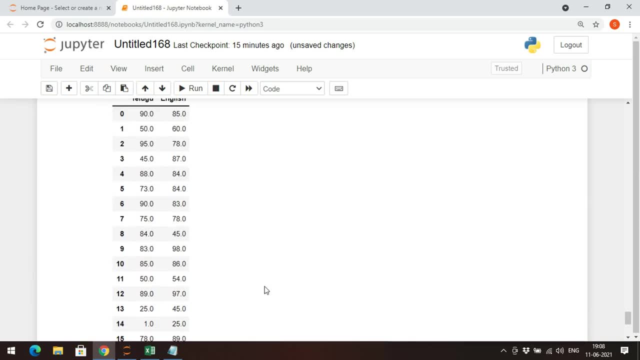 we are having some 45 because, eighth row, the english marks were missing. so, eighth row, the english marks were missing. right, so be here, you can observe here. so like this: uh, we can create 13th, 13th row, we can observe, the english marks were missing. 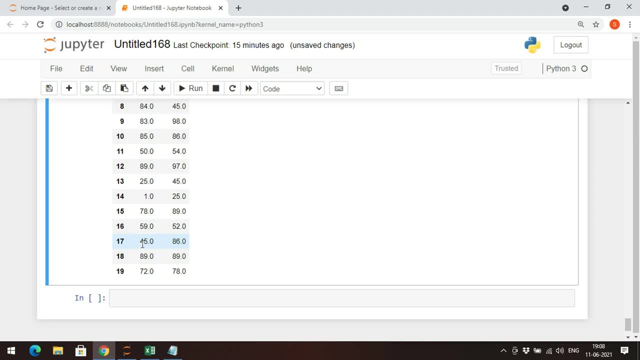 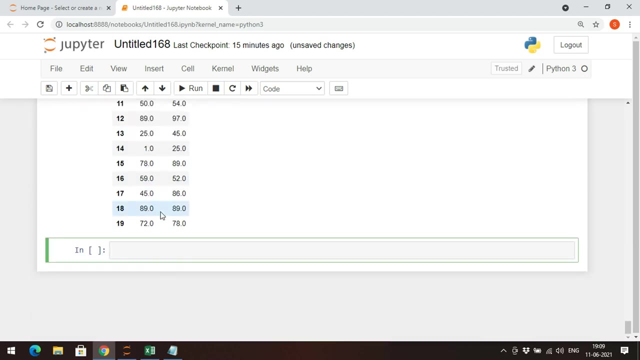 and similarly 17. the telugu marks were missing. so the normal value has been given and if you want to fill with the average value, average value, so then also you can go with this one. so directly we can apply if you want to give average marks for telugu, so df dot. 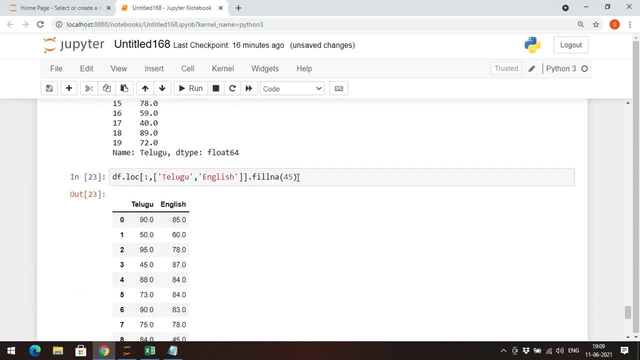 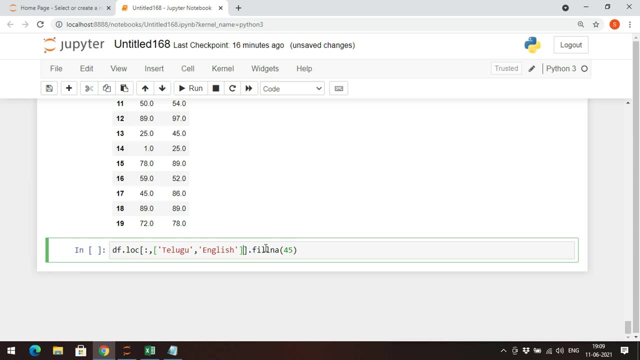 sorry, we can, we can apply here itself, right see, i'll just copy here and go with here. and i just want to apply the average marks. the average marks df of telugu, fill na, and here again go with df dot, sorry, df of telugu dot mean. we know the mean. there is a function called mean df dot, telugu dot mean. 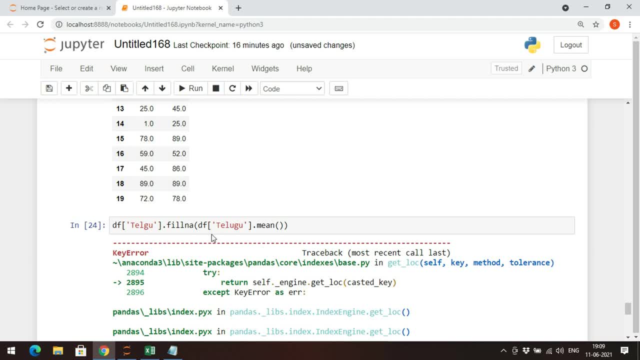 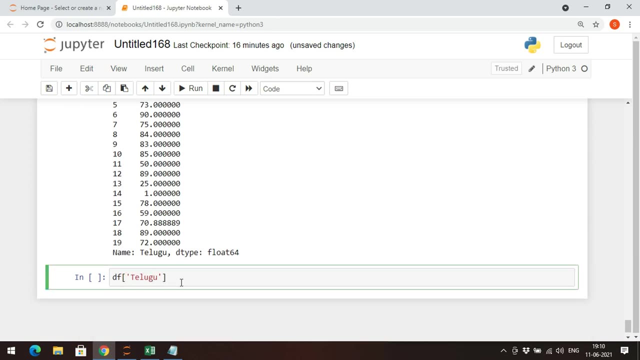 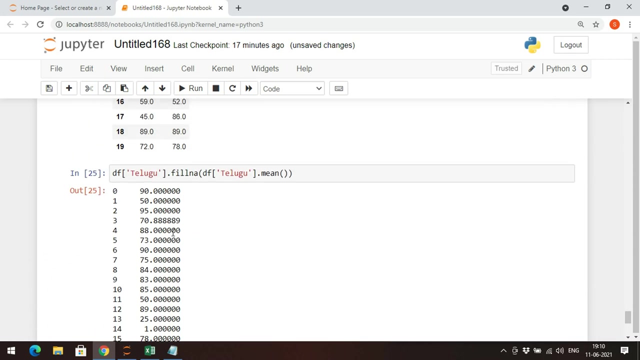 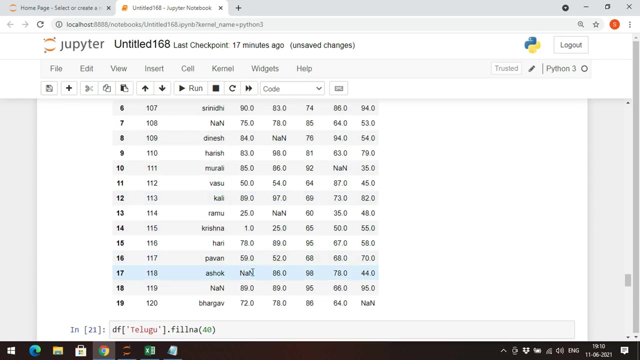 okay, automatically it will be executed just a second second. so see here again. you can see the average of the vos. that's right. df plus df, dot means so you could also see that there was this important section in the range, correct? so in the range of the balance. and then the Question. 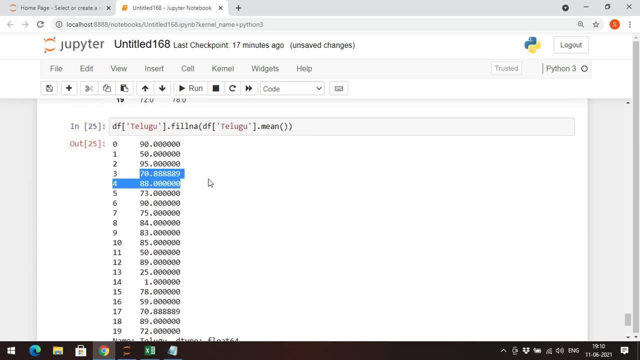 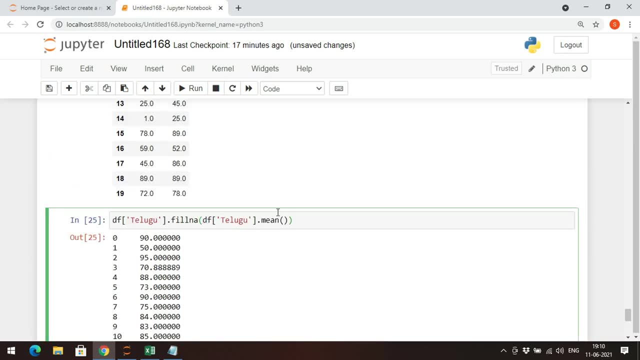 third row will be filled with the mean value. okay, and 17th row was also filled with the mean value. and if you don't want to use this one, so simply use a floor function. simply use the floor function so that we'll get clearly. so import math and here you can observe math. dot. floor of. 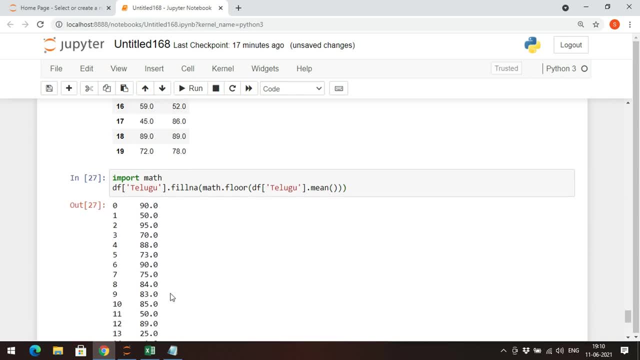 you can observe the clear value. so 70 is the average value for telugu marks. so you can get 70 value filled with both, filled in both the third row and the 17th row. so like this we can apply the formula and we can fill with the default values. and here also the second parameter is nothing. 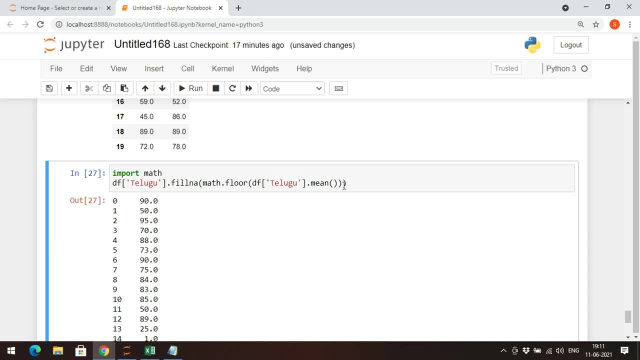 but an in place. so if you give that in place as true, automatically the original data frame will be reflected. so unless you give the in place is equal to true, the original data frame will not be reflected, but the new data frame will be created, right? so these are the two ways we can handle the missing data. so one is to remove the missing data. remove. 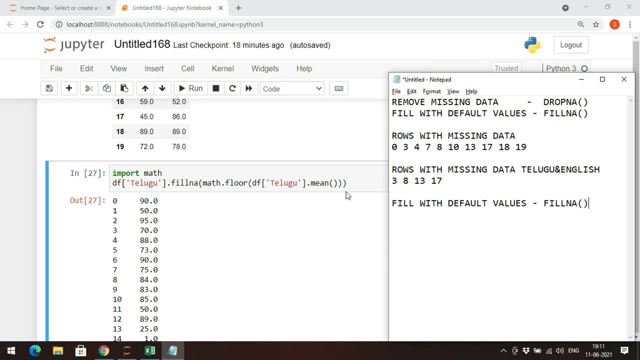 the data by using the drop na, and the second one is fill, with some default values using fill na. right, so hope you understood this one. let's stop here, and if you are having any doubts regarding this drop na and fill na, feel free to post your doubts in the comment section. 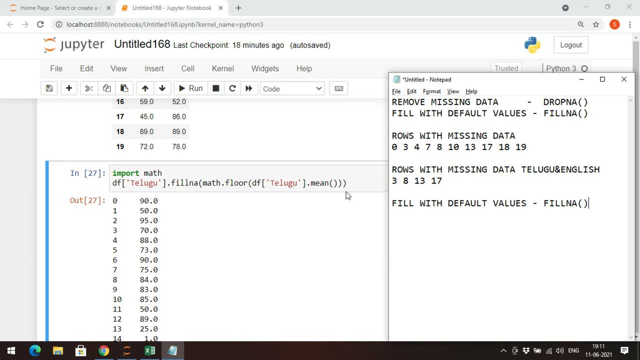 the will try to clarify all your doubts. if you really enjoyed my session, like my session, share my session with your friends and don't forget to subscribe to our channel. thanks for watching, thank you.